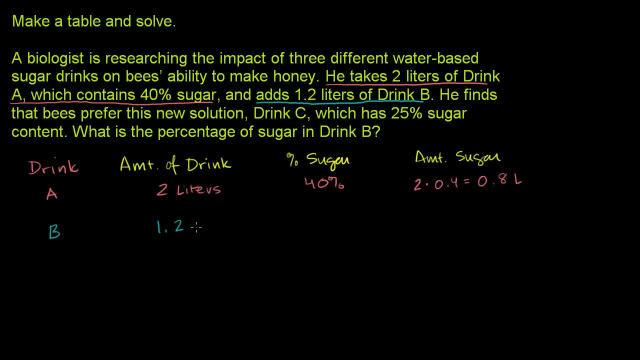 So drink B. he adds 1.2 liters of drink B. He finds that B's prefer this new solution. drink C. So when you add these two together, you end up with drink C. And we end up with how much of drink C. 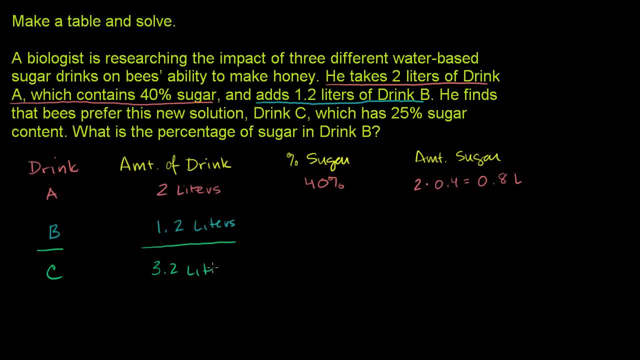 2 plus 1.2 is 3.2 liters of drink C, which has 25% sugar content. So this is 25% sugar, which also says we know the amount of sugar in it, Because if we have 3.2 liters of it and it's 25% sugar or 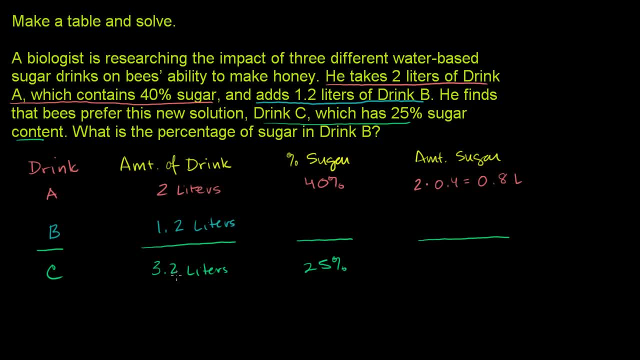 it's 1 fourth sugar. That means that we have 0.8 liters of sugar here. So this is 0.8 liters of sugar. Well, that I already wrote in the column name. That's the amount of sugar. It's 25% sugar. 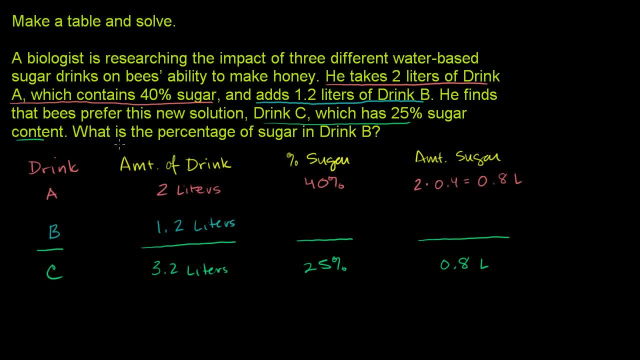 We have 3.2 liters of it. Now they want to know what is the percentage of sugar in drink B. So let's just call that x. So the percentage of sugar in drink B, Let's just call that x. So that's right over here. 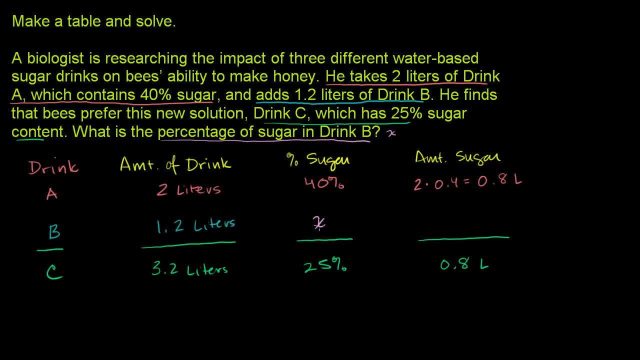 Now, if it's x% sugar here, or this is the decimal equivalent, that's x, How much sugar do we have? We have 1.2 liters times the decimal equivalent of sugar. So this is going to be 1.2 times x. 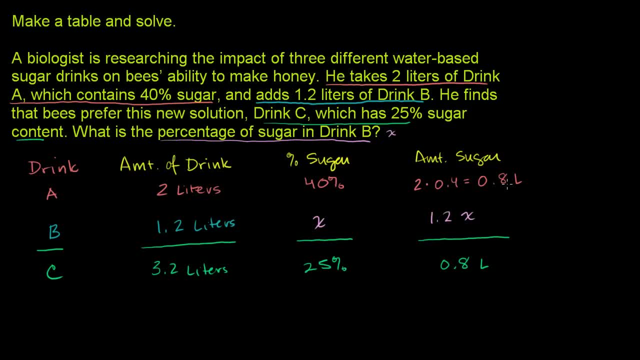 Now let's think about it. We have 0.8 liters of sugar in drink A, And when you add this amount to it, you still have 0.8 liters of actual sugar in drink C, So this thing has to be equal to 0.. 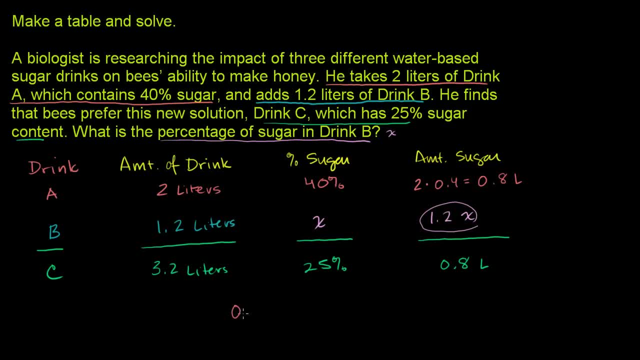 I mean we could set up an equation here. We could write: 0.8 plus 1.2x is equal to 0.8.. You subtract 0.8 from both sides, You get 1.2x is equal to 0.. 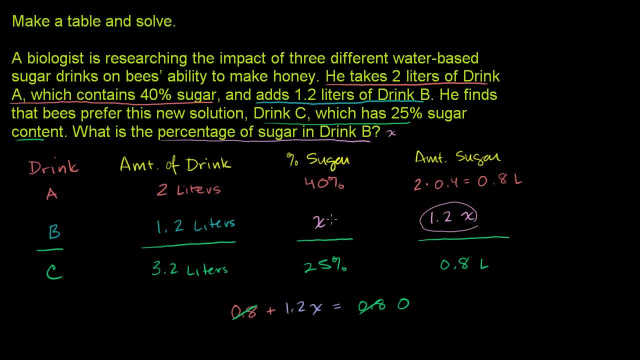 x has got to be equal to 0. So this thing right here has got to be 0.. There's no sugar in drink B, It's just got to be like 1.2 liters. I guess The solution is. The solution is water. 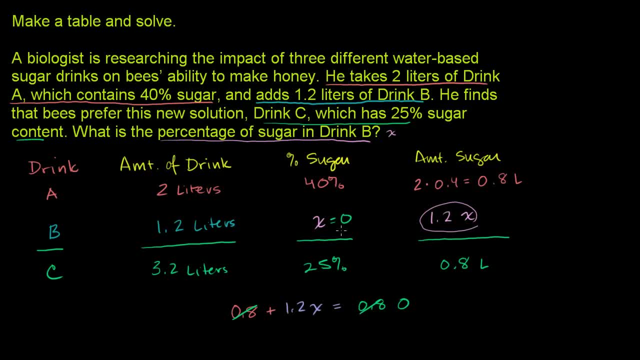 So it's 1.2 liters of water. There's no sugar in drink B. It is 0% sugar. 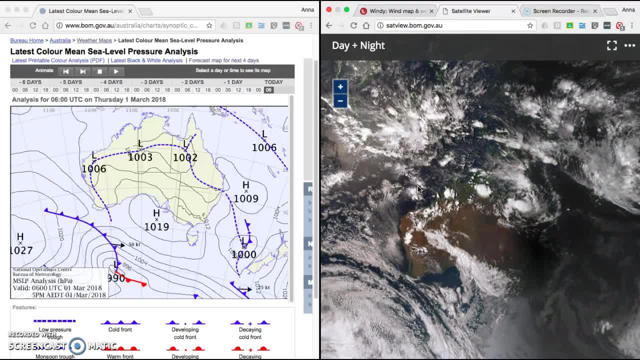 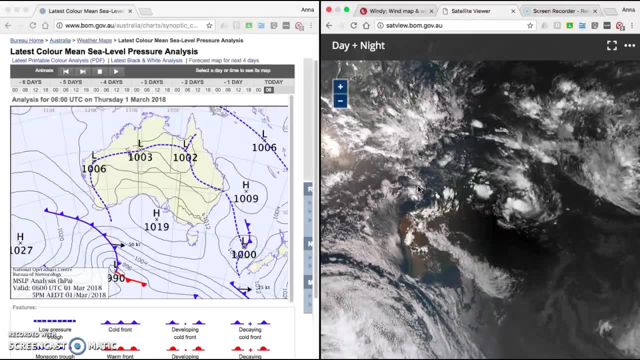 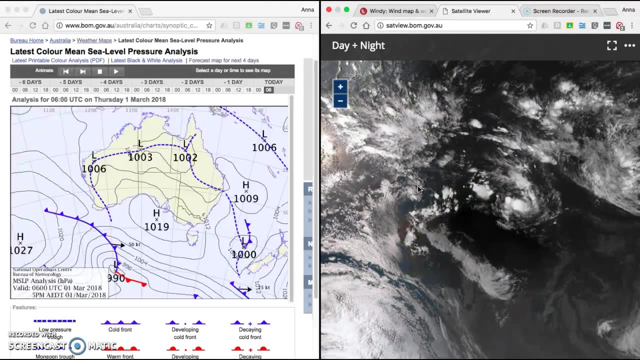 Okay, boys. so what I'm going to show you today is how to read a synoptic chart and what all those lines and squiggles and things mean. And once you know that, you know, you'll be able to- hopefully, by the end of this, to predict the weather. Okay, so, on my left and on your left, with what I'm circling, 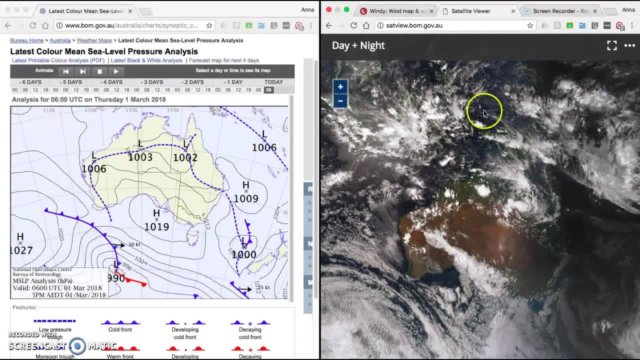 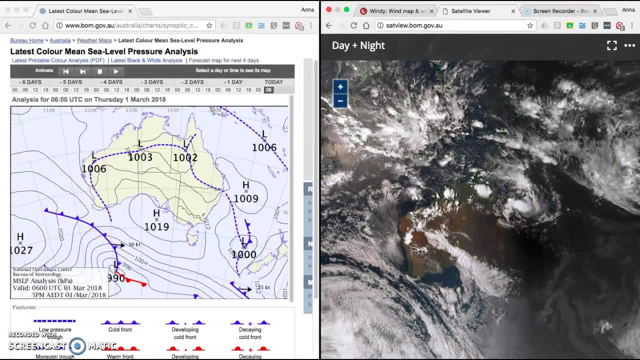 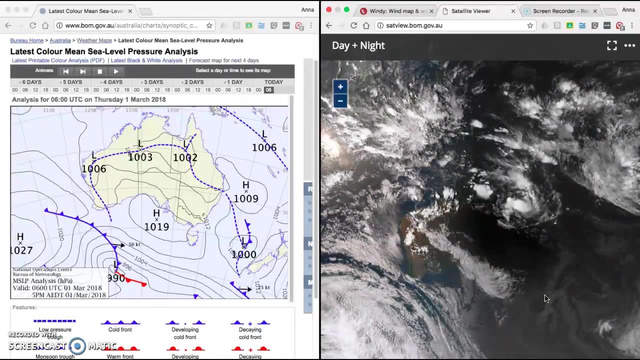 right now is a synoptic chart and on my right is a satellite image, So I'm going to show you a few of them, and it's good to have them side by side for you to understand what's happening. This is real time. it's satellite image, Okay, so this is Thursday, the 1st of March. Okay, and it goes for. 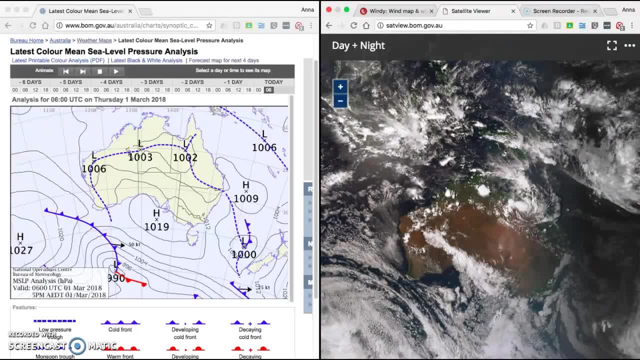 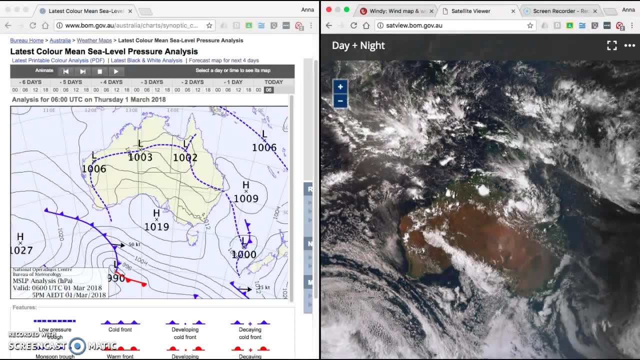 three hours. You can get this on Bureau of Meteorology. I'm going to stop at about six o'clock or maybe I'll go back to 5 pm. Okay, I'm going to go 5 pm because this is the time the synoptic chart was from, So you can see. 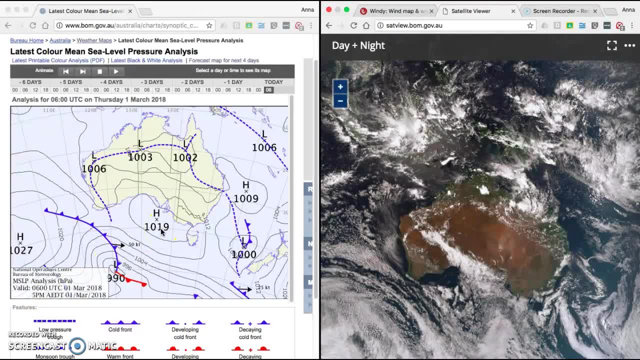 here it says 5 pm. Okay, so let's look at our synoptic chart. We can see that there's just there's a variety of different lines on here, But the most important one that I want to point out right now is an. 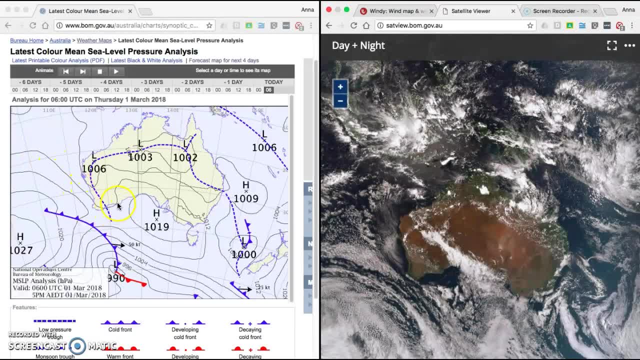 isobar. So this black line, this black unbroken line, it's called an isobar. An isobar measures places of equal pressure. So here it says 1012, so that's 1012 hectopascals. And so on this line, anywhere along this line, it's 1012 hectopascals, Anywhere. 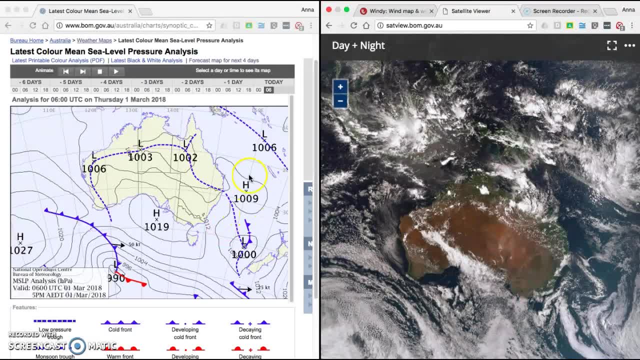 along this line if I follow it. well, that's a bit of a failure because it doesn't actually have the number, But I know here's 1012,, here's 1004, so it shouldn't be the number in between. So it's.